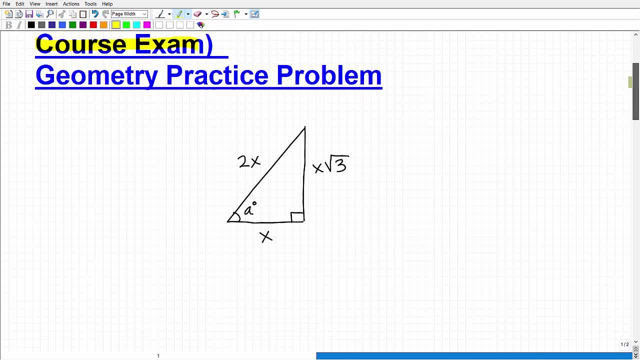 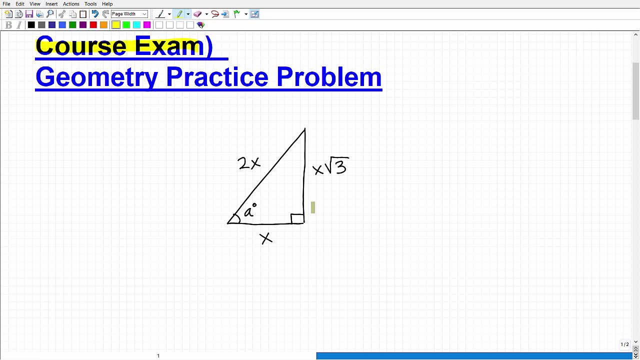 being said, I'm going to go ahead and start the video. So, with that being said, let's go ahead and check out this problem. Okay, so here I have a right triangle. Now, before I say anything else, I am going to solve this problem, but I'm going to give you an opportunity for you to think about it And, you know, hopefully you can try to figure it out. But then I'm obviously going to give you a hint and then I'm going to solve the problem. Okay, so we have a right triangle and we have some lengths here. We got x and x, square root of three, And then we have two x. So I want to 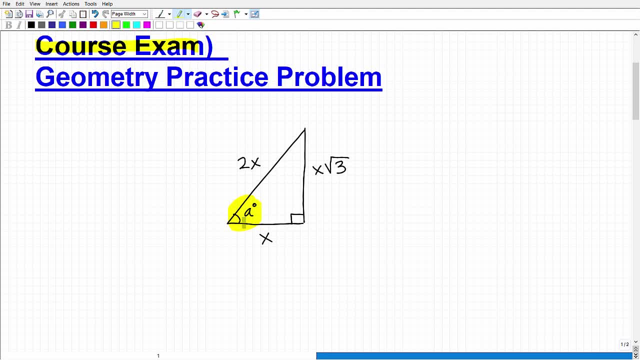 know is: what's the measure of angle a? How many degrees is angle a? Okay? so for those of you out there, I think you know how to solve this problem. I would pause the video and go ahead and do it. All right. Now, for those of you who think that you need a hint, okay, I'm going to give you a hint. Okay, so we have a right triangle. This is really, really important. Now, when we're talking about right triangles, we're going to talk about right triangles. 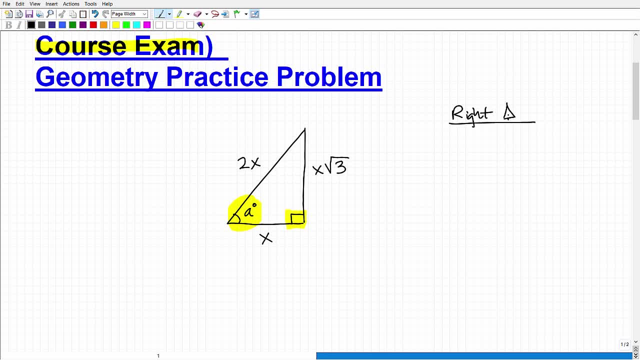 triangles. all right. what did we learn about right triangles? Well, in geometry, okay, obviously you learned the Pythagorean theorem. all right, a squared plus b squared- let me just kind of get rid of that- equals c squared. okay, but that has to deal with the lengths of right triangles. so 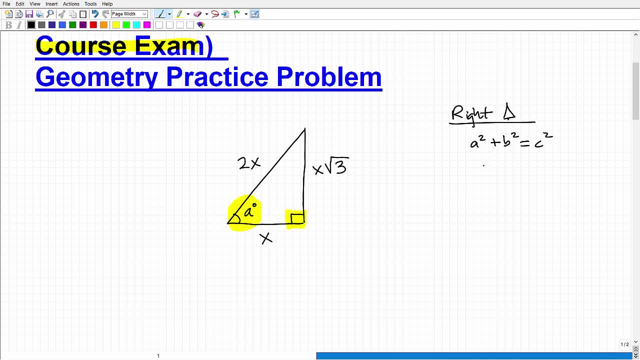 I'm asking for an angle, so that's not going to really help me out. and then also you learn some basic trig, so sine, cosine and tangent. okay, so these are particular ratios in a right triangle that have to deal with angles. so this could definitely help you out, but we don't have any. 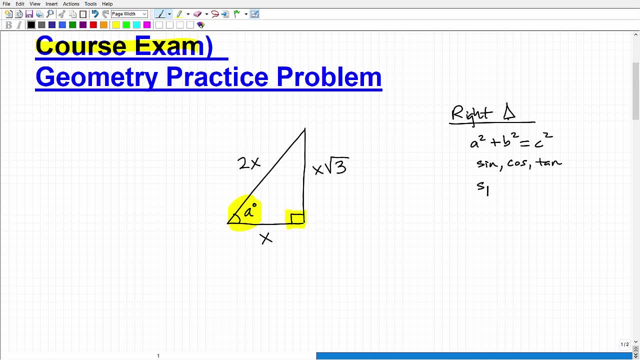 actual values here. and then you learned about special right triangles. Now right triangles- you learn more about right triangles as well, but these would be some of the things that you might be thinking about. I would kind of hone in on. what did you learn about special? 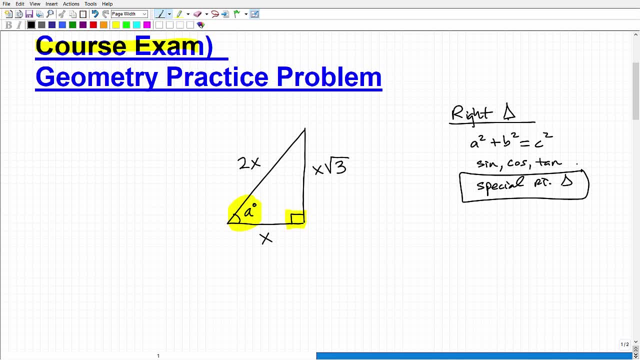 right triangles, Right triangles. okay, all right. now there are two different type of special right triangles in particular that we kind of cover in geometry because they come up all the time. so the first is 45,, 45,, 90, okay, these are degrees. that's one special right triangle and the other is 30,. 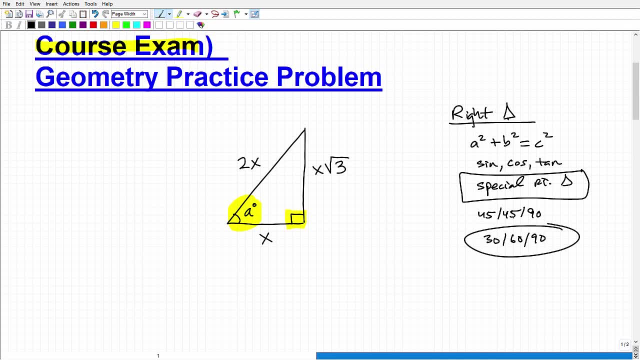 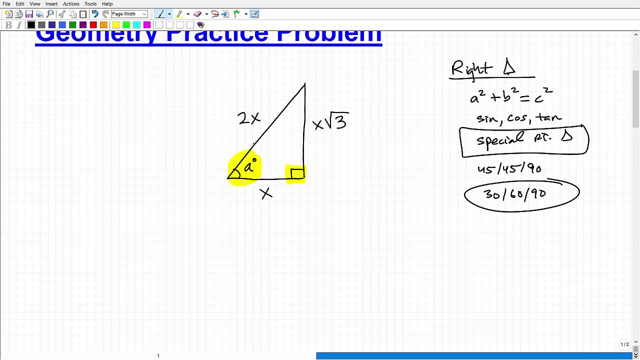 60, 90,. okay, and that's this situation right here. okay, 30, 60, 90,. you need to understand that How the angles and lengths of a 30, 60, 90 right triangle work. so let's go ahead and let me just 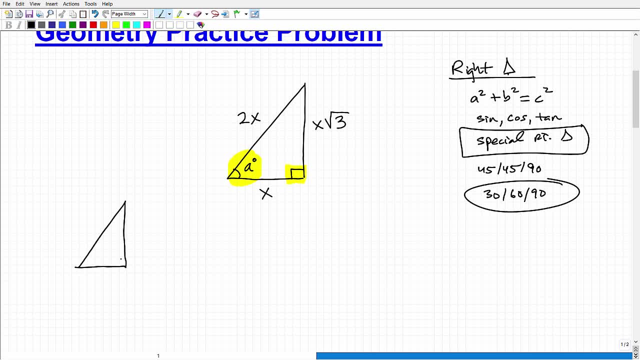 sketch a basic 30,, 60,, 90, and here's the rule. okay. so here, this is obviously the shortest side, okay, of a 30,, 60,, 90,. this is the longest side, and then this is the middle side. so let's. 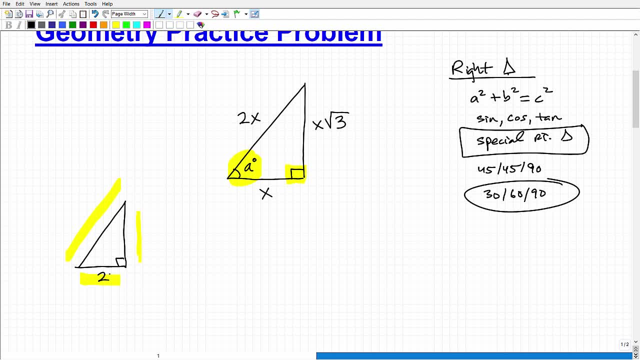 say I had the shortest side was a length two. okay. now, if you recall, this is a 60 degree right here, okay. so this is 90,. this is 30, right here, okay. the hypotenuse is always going to be double, whatever the shortest side is. so what's double of two? that's four. 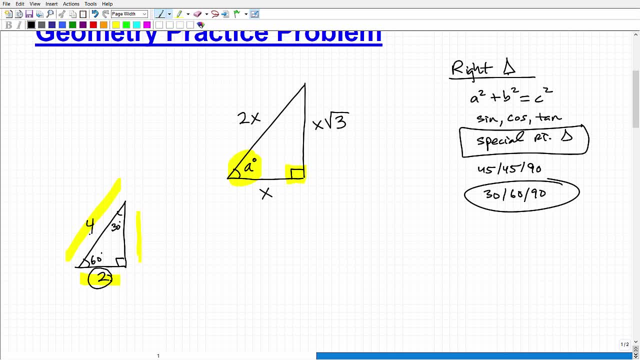 right twice or two times. the shortest side is the hypotenuse, okay, and the middle side is going to be whatever. the shortest side is times the square root of three, so that'd be two square root of three. so you want to know these lengths. 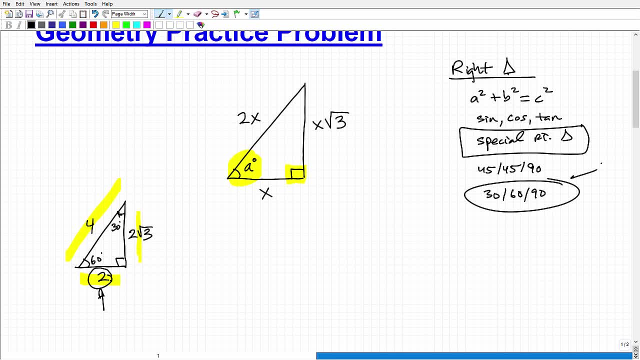 and these angles, okay for 30,, 60,, 90, and you kind of. you know a lot of this. this type of problem is very common, right? so if you look here, just look at the pattern, here I have the shortest. 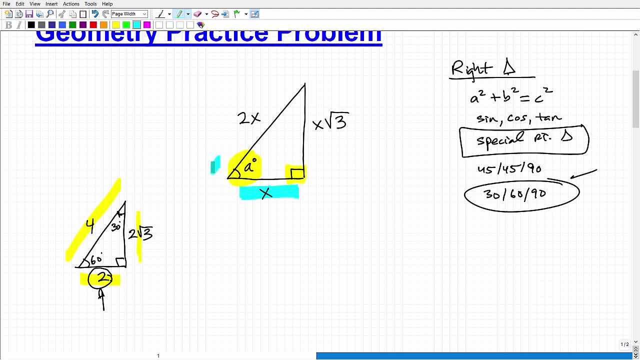 side x. so if you look at the hypotenuse, it's twice the shortest side, so it's 2x. okay, so it fits our pattern. and then here that middle side is going to be the shortest side times square root. 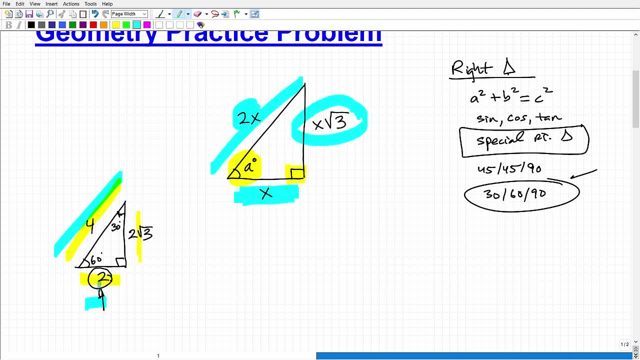 of three. so because these lengths are in the ratios of a- 30,, 60,, 90,- we can determine the hypotenuse and we can determine that a is what it's: 60 degrees. so angle a is 60 degrees. 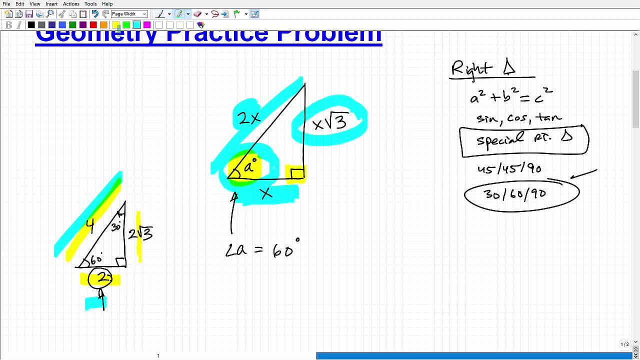 all right. so hopefully that was pretty easy. and now you know, a lot of you out there might be like, oh, that was, that was easy. well, everything's easy when you know what you know what you're. 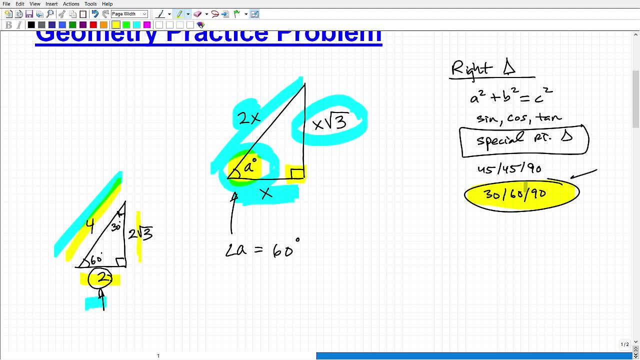 doing if you will, right. but if you struggled with it and you kind of use some of these other things, you know, that's good too, because at least it got you thinking about what you know about right triangles. but these special right triangles, they come up a lot in any geometry-related type of 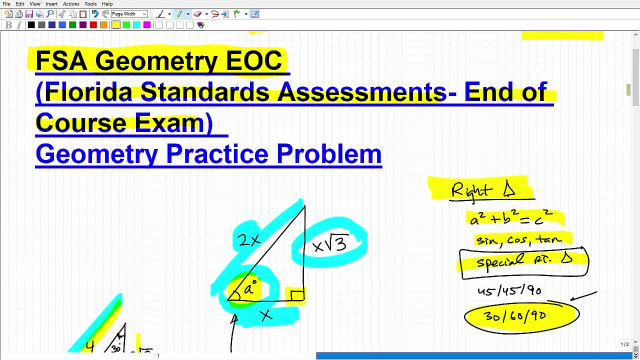 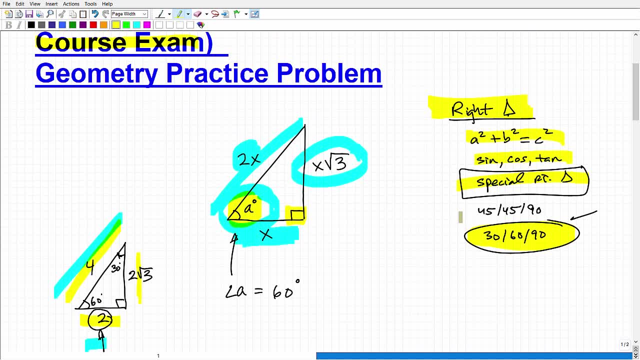 test not only FSA, geometry, EOC, but things like the SAT or ACT, etc. so really, you know, make sure you understand these special right triangles: 45,, 45, and 30,, 60,, 90, and, of course, 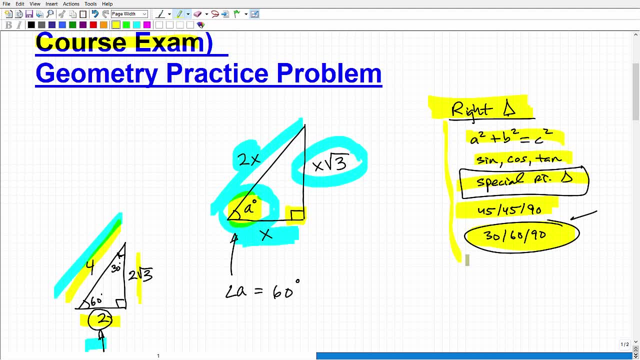 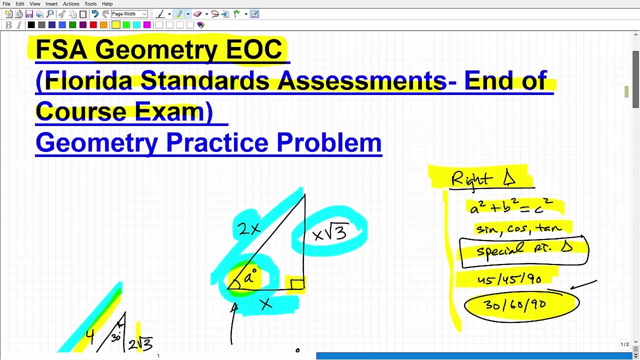 I could cover a lot more about right triangles and huge topic in geometry, but you know we're going to keep this video kind of short, all right. so again just a quick pop quiz on something that might come up. so if you got this right, that's excellent, okay, but by no means is 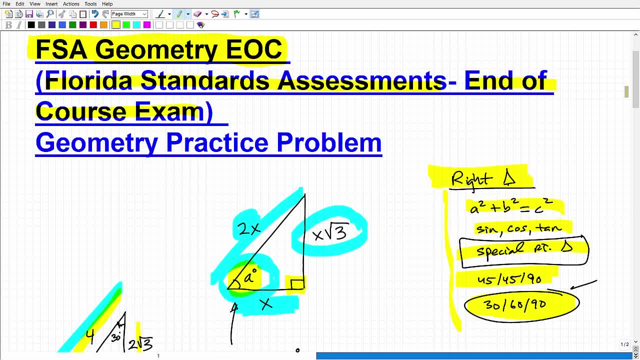 that verification that you're ready for the entire. you know, FSA, geometry, EOC- there's a lot of topics covered in geometry. now, if you didn't get this right I wouldn't panic, but you know, use this. 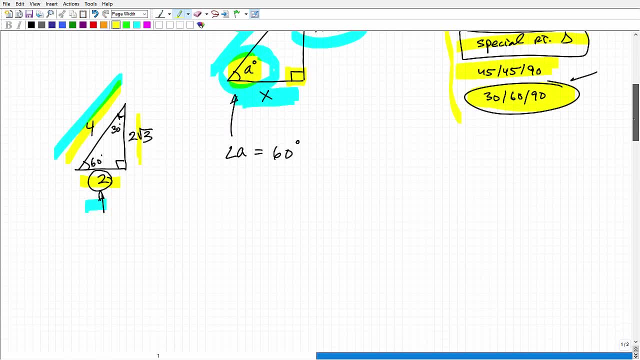 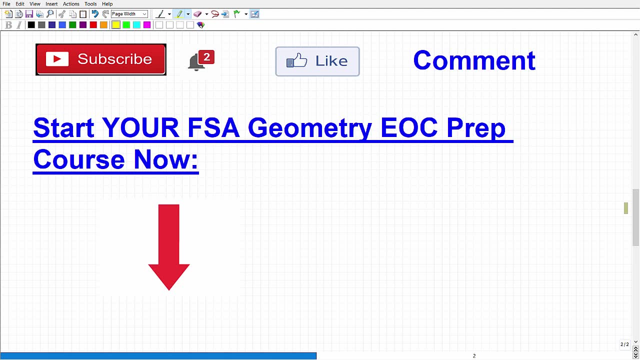 as feedback to you know, you know to make some changes, so let's go ahead and wrap up this video. so the first thing is I always stress to those of you watching my videos for particular tests is always start with your teacher and whatever material that they're telling you to. 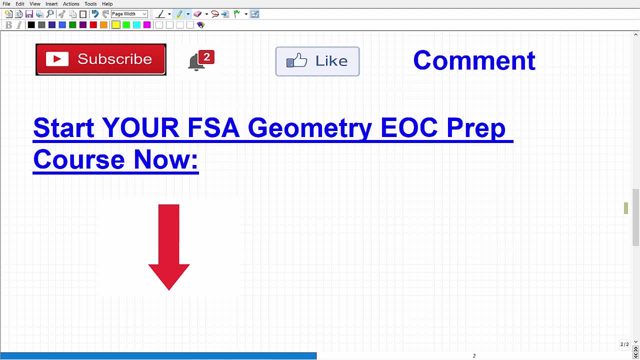 study. okay, always start there. as a teacher, I know what it's like. hey, you're telling your students, you're giving them the best advice and guidance because you know they're right there trying to help you. so you know before you kind of make up your own study plan. you don't want to. 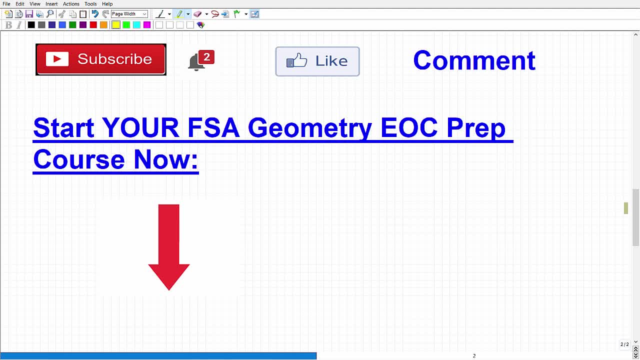 do that. you want to maximize everything that your teacher is offering, but if you need a supplement beyond that, a course like mine would be excellent. so, again, I'm going to leave the link to my FSA geometry EOC prep course. 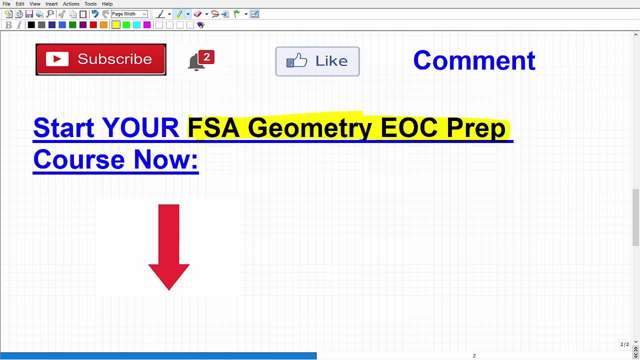 super comprehensive. I think you'll be impressed with it. okay, because I've put a lot of work, many, many years, to build this thing out, so it's going to be pretty much on par probably, what you're getting in your class. so, again, I'm going to leave the link to that in the description of.